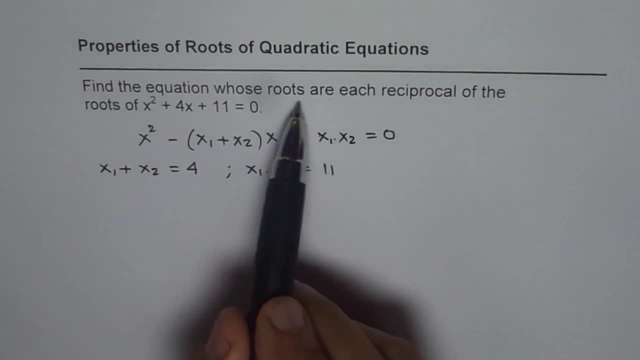 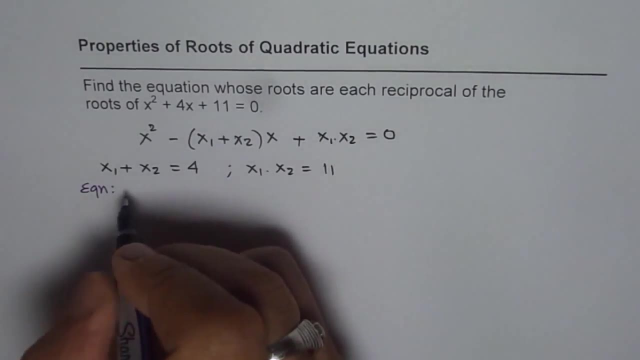 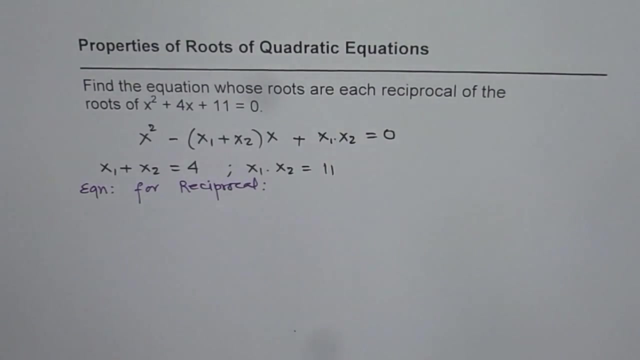 Now the question here is: find the equation whose roots are each reciprocal. right, So we have to find a new equation. So we say equation for reciprocal, Reciprocal roots. What does that mean? It really means that the roots of the second equation should be 1 over x1 and 1 over x2, right, That is what it means, correct? 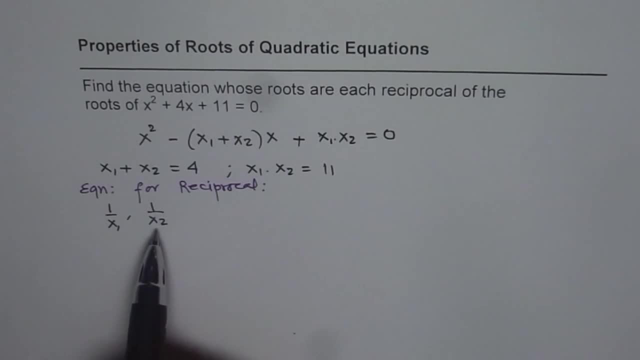 So now let the roots be 1 over x1 and 1 over x2.. Now the strategy is to find sum of these and product of these, then write it in the quadratic equation form. That is how we are going to use properties of roots of quadratic equations. 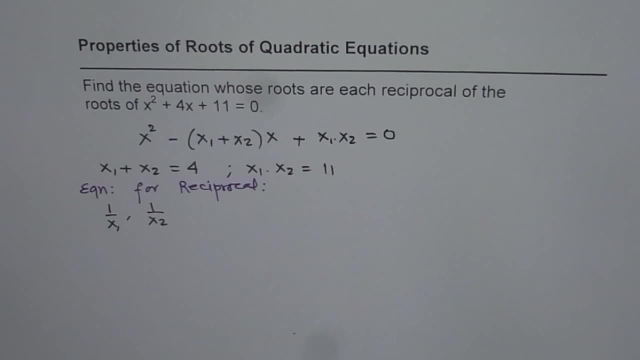 I think everything comes together now, right. So let us first find this sum. So what is sum of 1 over x1 plus 1 over x2?? So it is. we will take x1, x2 common and it becomes x2 plus x1.. Now we know x1 plus x2 is 4 and the product is 11.. So we get sum as 4 over 11.. 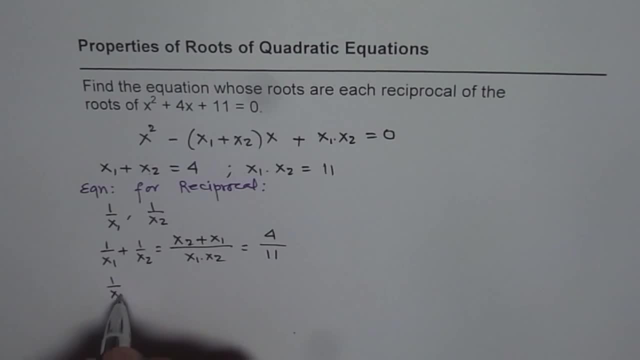 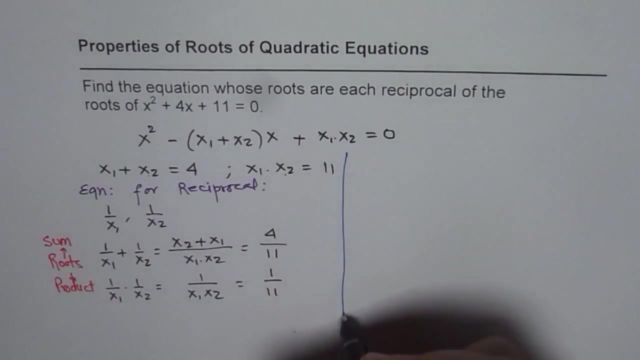 How about the product? That is 1 over x2.. x1 times 1 over x2.. So the product is 1 over x1, x2.. We know x1, x2 is 11.. So the product is 1 over 11, correct? So at this stage what we have gone here is we have got sum of roots right And we got product of roots correct, So we have both the equations. Now we can write down our quadratic equation in this form, which is 1 over x1 times 1 over x2.. 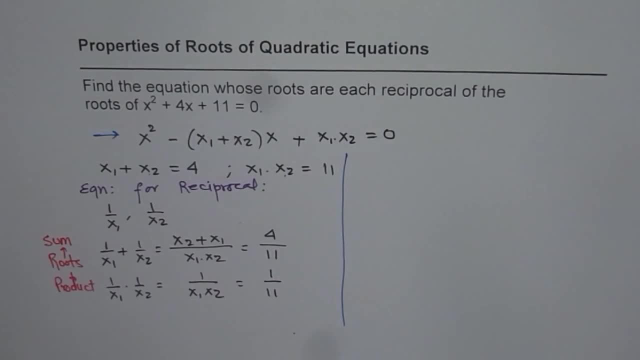 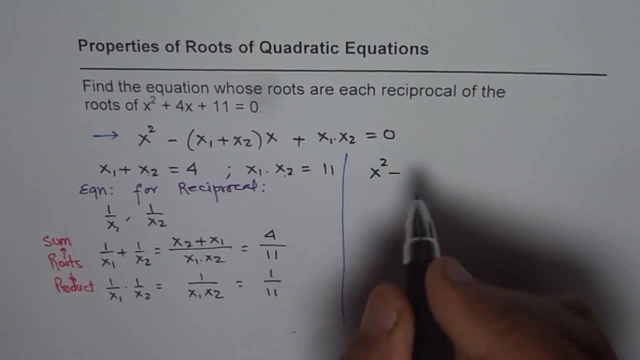 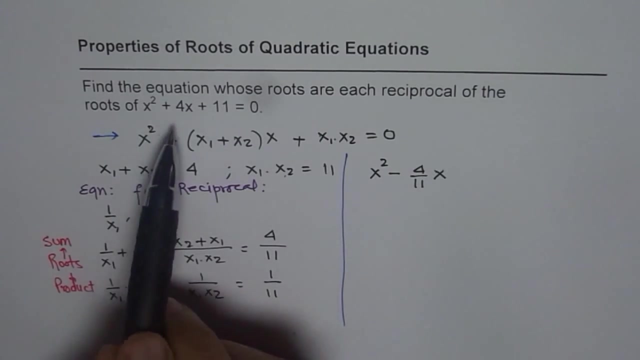 Which includes sum and product form. correct, So we can write our equation as x2 minus. what is the sum? 4 over 11, right, So we have 4 over 11x And this we did a mistake here And the mistake is this should have been minus 4.. So let me correct this. It is not late either.